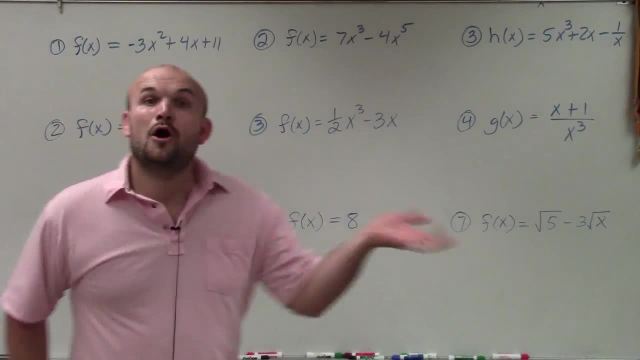 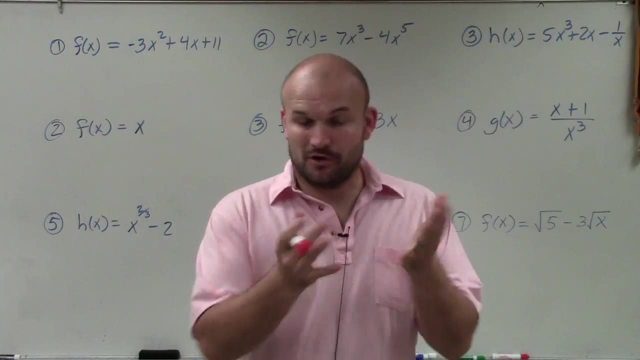 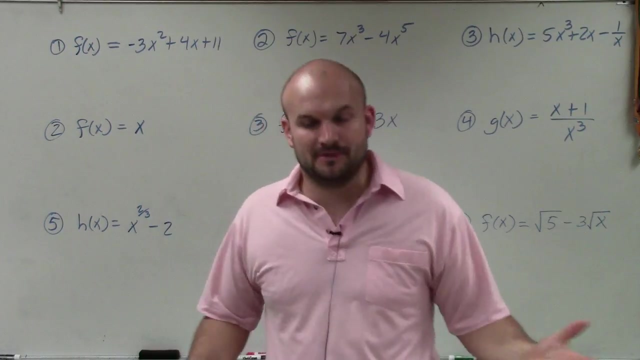 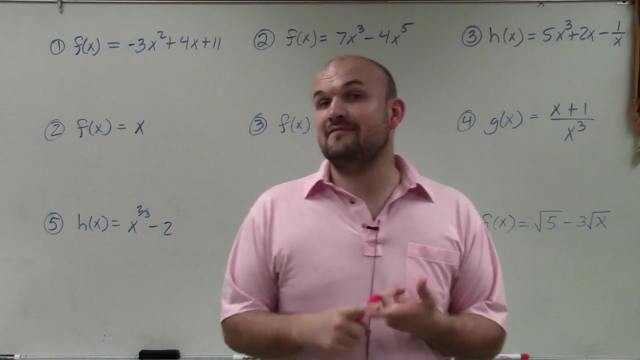 Welcome, ladies and gentlemen. So what I'd like to do is show you how to determine if a function is a polynomial function or if a function is a polynomial. So, basically, the way to determine if a function is a polynomial is basically looking at two rules. We have to make sure that all of our variables have powers that are one non-negative integers. That means our all of our variables have powers that are one non-negative integers. 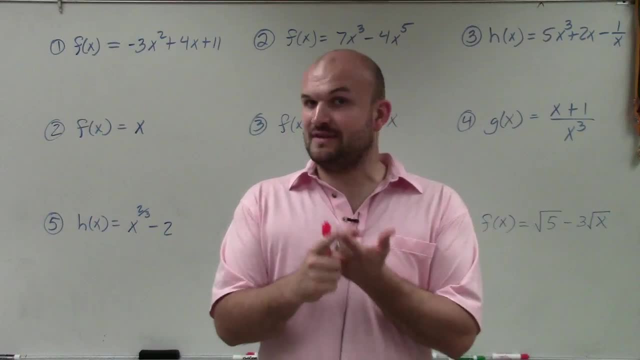 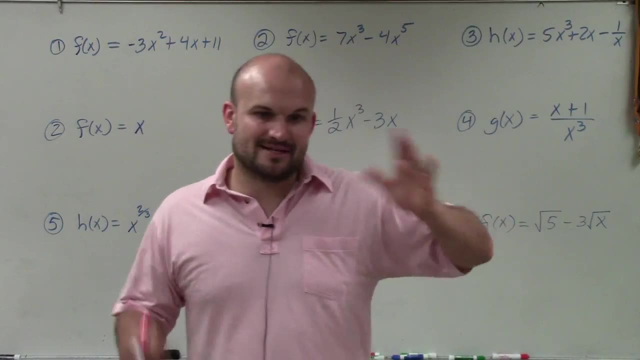 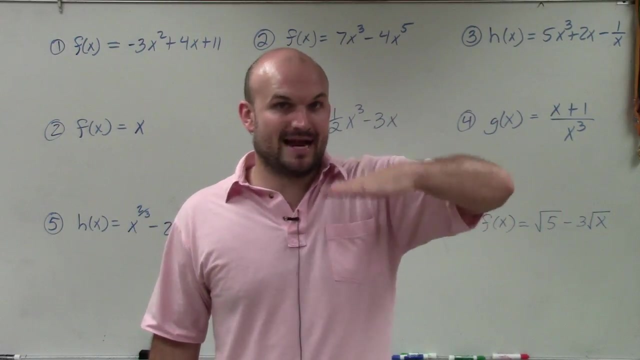 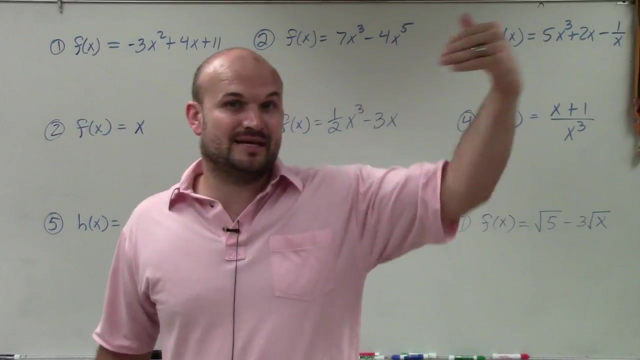 That are non-negative integers, meaning they have to be positive, they can't be negative And they have to be integers. that means they can't be fractions and so forth. This also works in the same respect. you know non-negative and integers also helps out. remember, like square roots and radicals, We can rewrite those as fractional exponents. So be careful, So you also can't include any of your variables to be under a root, positive or negative, As well as remember negative powers mean. 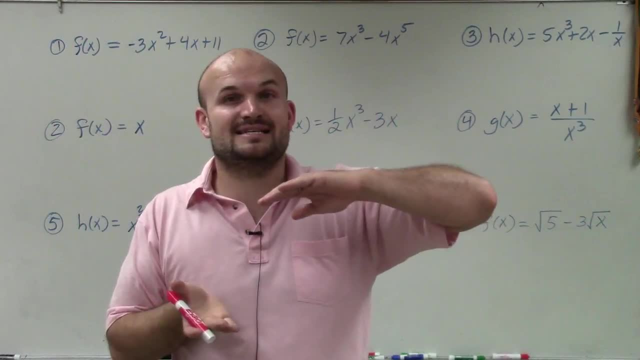 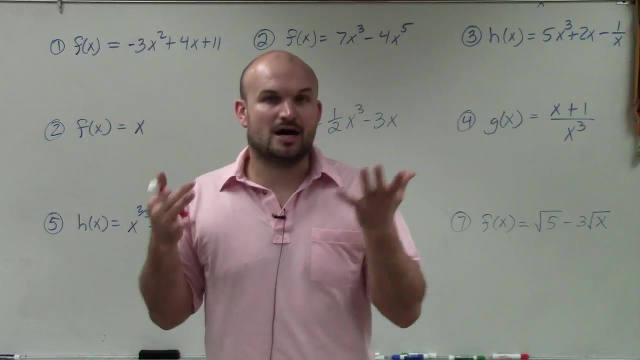 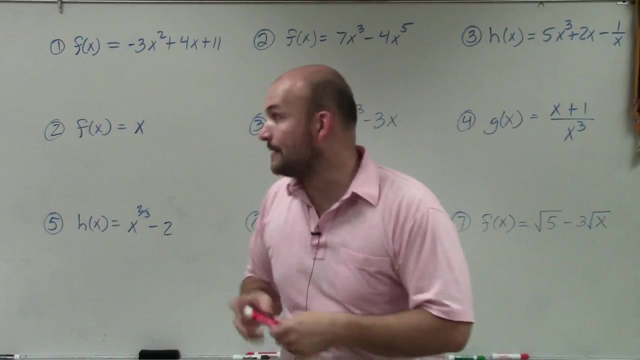 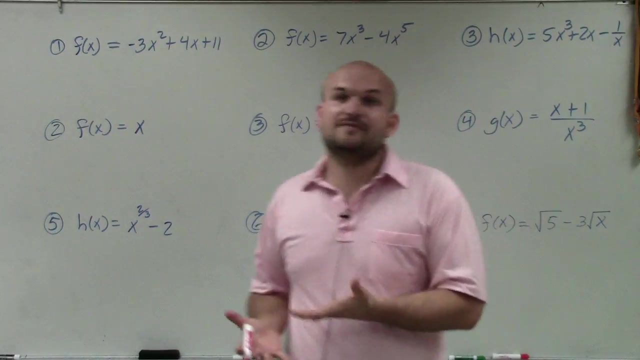 basically mean that the variable can also be rewritten as in the denominator. So you also cannot have any variables in the denominator. Okay So, but the overall really definition is you, the powers of all, the powers of the polynomial of every exponent has to be non-negative integers. Okay, So when we look at this, basically, what we're going to do is look at every single term and make sure that we have a non-negative integer. So here we look at each and every term and you can see that the powers are two: one, 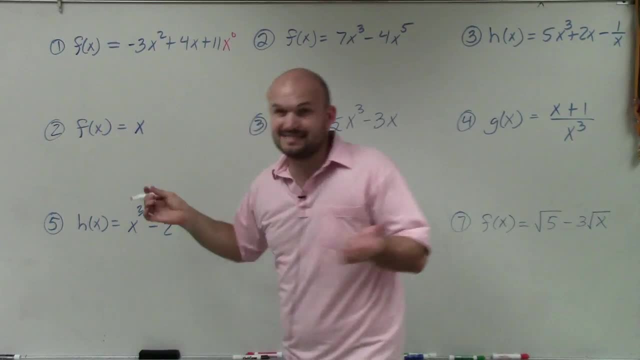 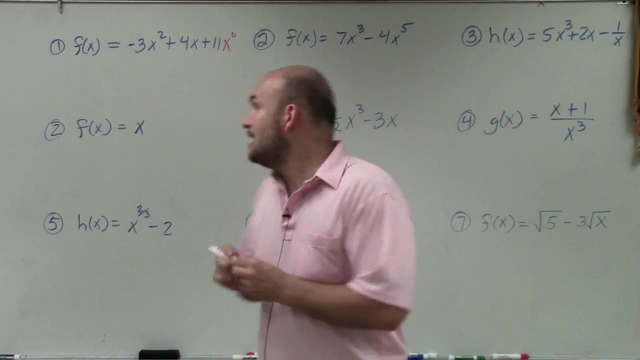 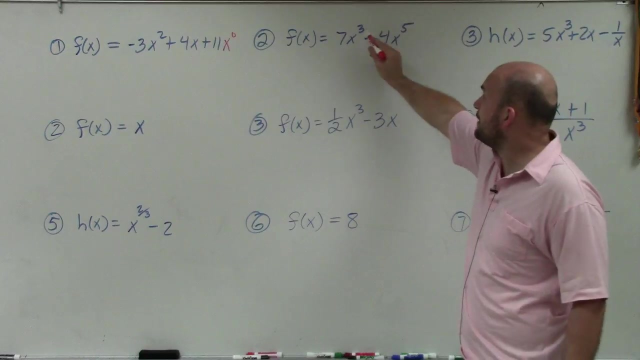 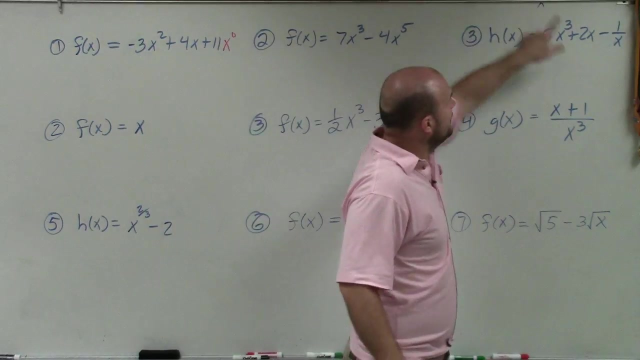 and this one you could write in x to the zero power, because x to the zero power is one. I'm not going to do that for every single one here, but that is that is important, which we'll come up to later, But anyways, this is an example of a polynomial function. Over here you can see that again, both of my powers are integers or non-negative integers. So that is an example of a polynomial function. Over here we have a problem, We, where the power here is not of a non-negative integer, because, yes, 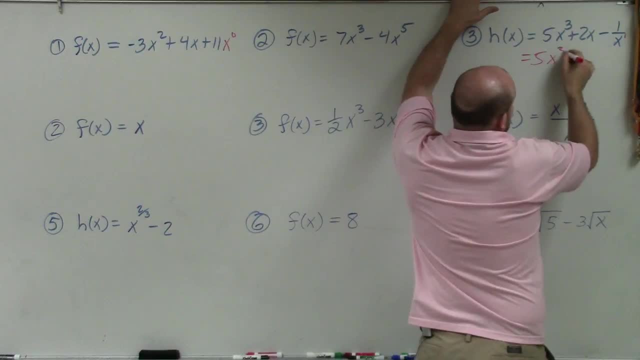 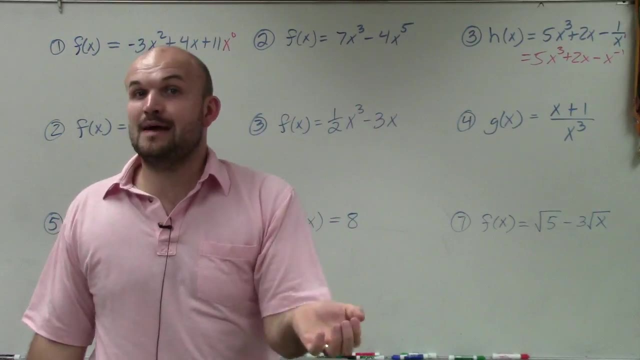 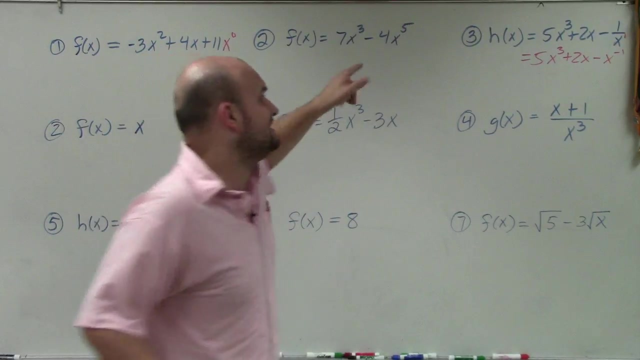 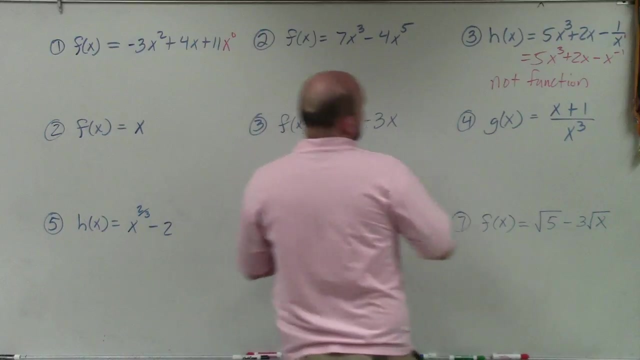 that's one up there. but really when we rewrite this five x cubed plus two x minus x, to the negative first, because when we rewrite and a variable in the denominator, we rewrite it as positive or rewrite it in the numerator, it's going to have a negative power. So therefore, that is, this is not a function or, I'm sorry, not a function. It can be a function, It's just not a polynomial. 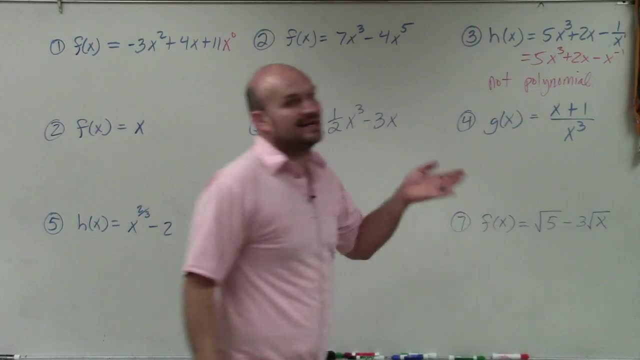 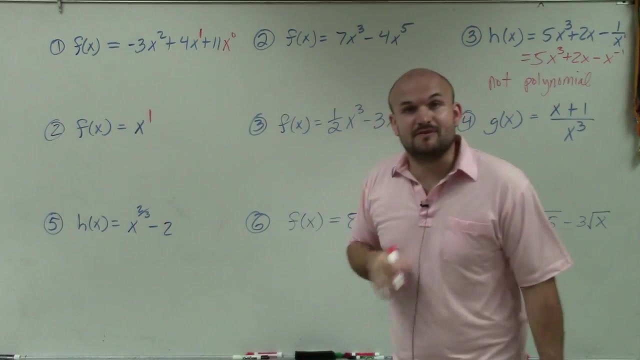 So anytime you see a variable in the denominator, it's going to be basically a non-negative power. So therefore it's not going to be a polynomial. let's go and look at this one Again. this one doesn't show the power. However, the power in this example is one kind of like over here. So that is an example of a polynomial function. 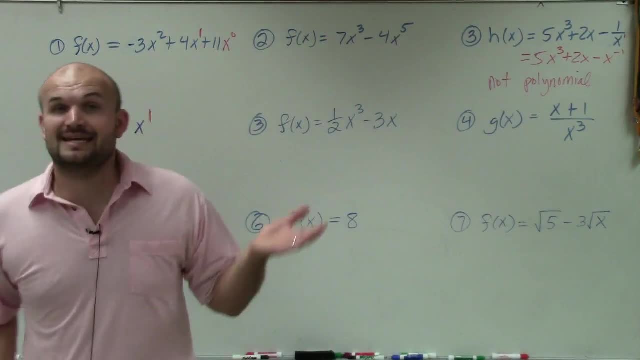 Okay, over here. Yes, we have a fraction, but that fraction is of- is the coefficient right, It's not the power. So therefore, again, we look at the powers. That's all we're going to have to do. So that's one up there. 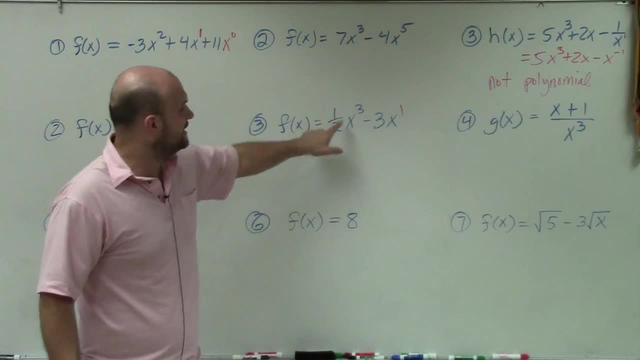 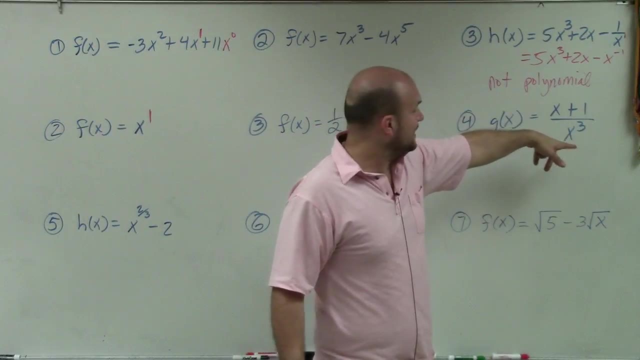 concerned about is the powers. We don't care about what's in front. So the power in here is 3 and 1.. So therefore this is a polynomial function. In this example again, you can see a variable here in the denominator. 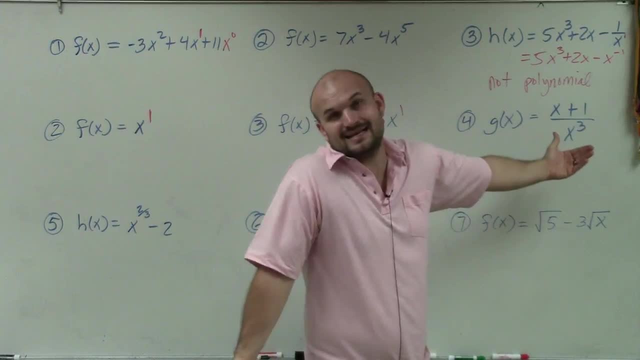 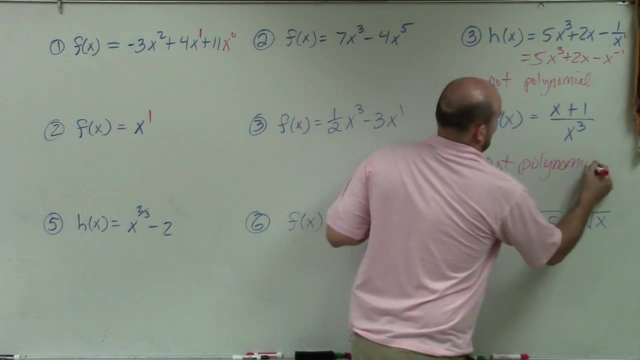 So therefore you can't have variables in the denominator, because that's basically a non-negative integer when you rewrite it in the numerator. So therefore this is not a polynomial Over here again, as I mentioned, non-negative integer Fractions are not integers. 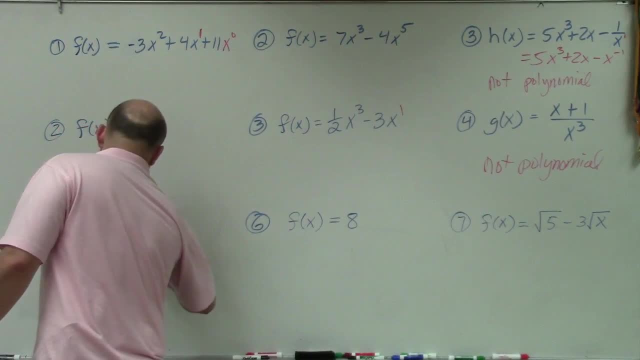 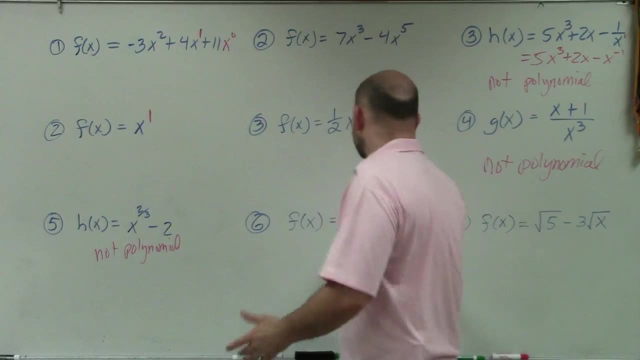 So this is an example of not a polynomial. Now this one gets a lot of students: f of x equals 8. This is a polynomial because, again, as I mentioned, you could still have a variable in here, just x to the 0 power. 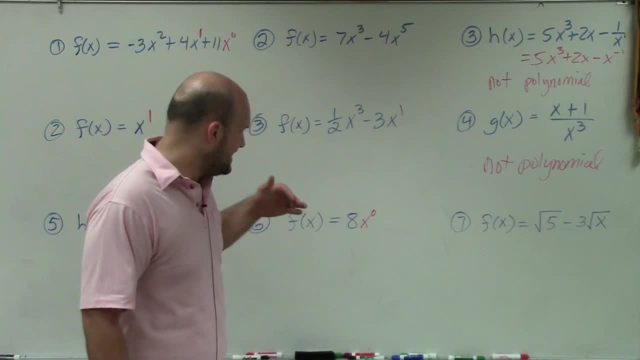 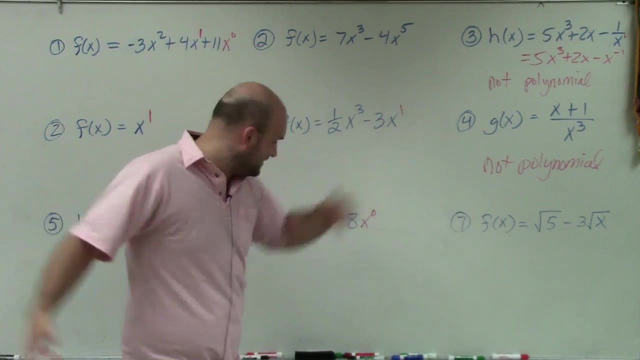 Well, 0 is an integer And it's not negative or positive, So it's not going to fall into being negative. So therefore, this would be a polynomial. because the power is going to be negative, It's going to be 0.. 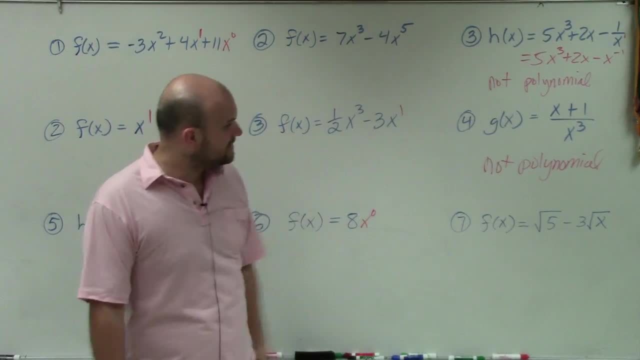 It's non-negative, which, of course, And it's also an integer. Over here you can see the square root. Well, the square root of 5, we know. oh, if that's OK, you can have that as a coefficient. 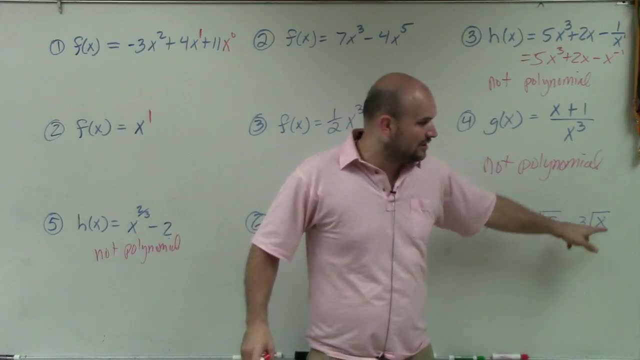 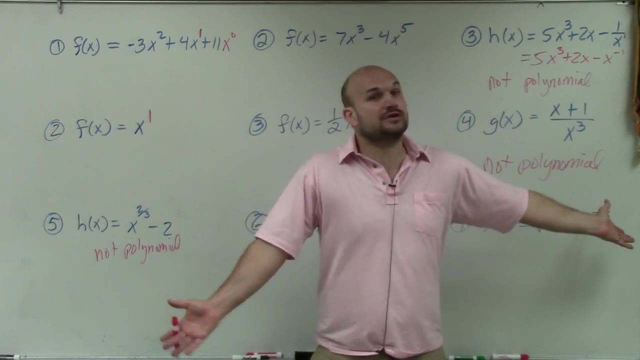 The only thing we're concerned about is the power. Well, we can't have a variable being under the square root or in the denominator, Because this would be rewritten as x to the 1 half if you were to convert that to a rational power. 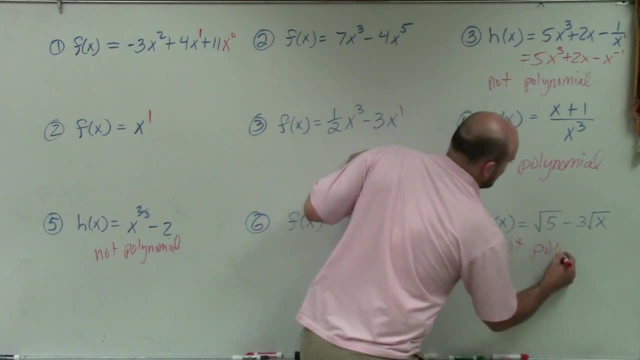 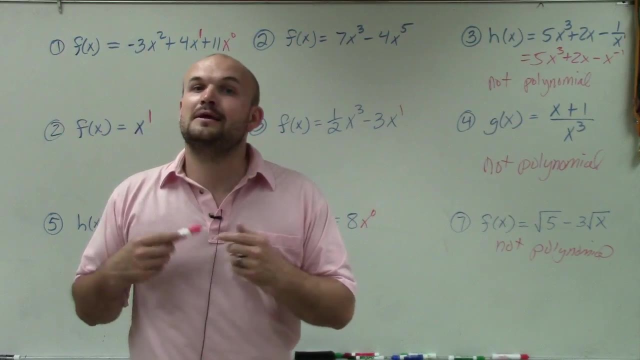 So, therefore, this is another example of not a polynomial. So there you go, ladies and gentlemen. That is how you determine if a function is a polynomial. Thanks, 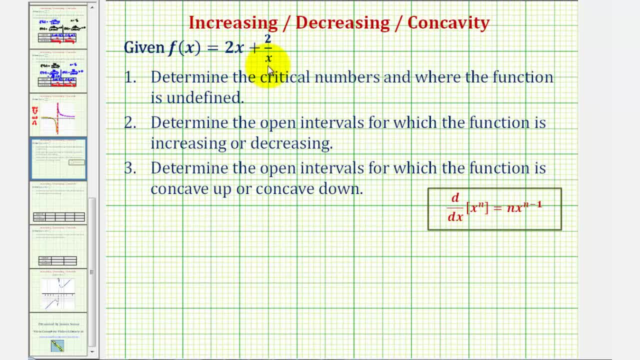 We're given, the function f of x equals two x plus two divided by x. Number one- we're going to determine the critical numbers and, where the function is undefined, Number two- we're going to determine the open intervals for which the function is increasing. or. 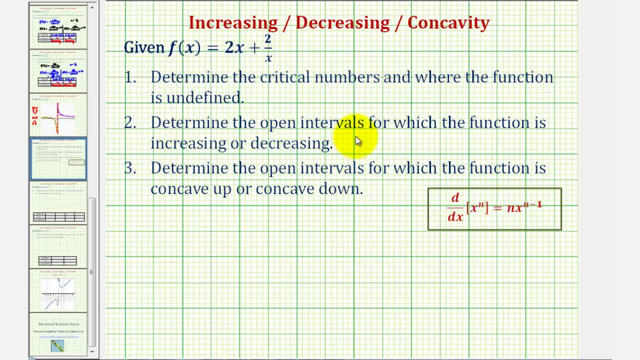 decreasing. And then, depending on which version of the video you're watching, we may also determine the open intervals for which the function is concave up or concave down. So, beginning with number one, we'll determine the critical numbers and, where the function is undefined, Looking at 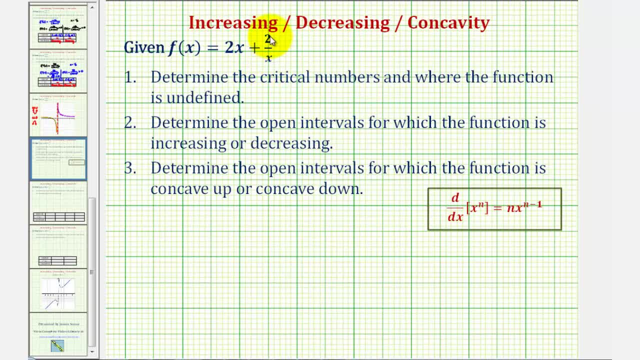 the function. notice how, when x is zero, we'd have division by zero here, which means the function would be undefined. So the function is undefined at x equals zero. Now to find their critical numbers, we'll find the first derivative and determine where that's equal to zero or undefined. 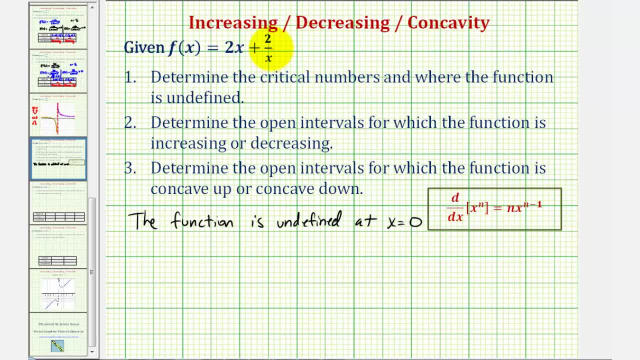 Before we find the derivative, though, let's look at the second term. here We have 2 divided by x or 2 divided by x to the first. If we move this up to the numerator, it would change the sine of the exponent, So we can write this as a derivative. Let's write this as equal to x.